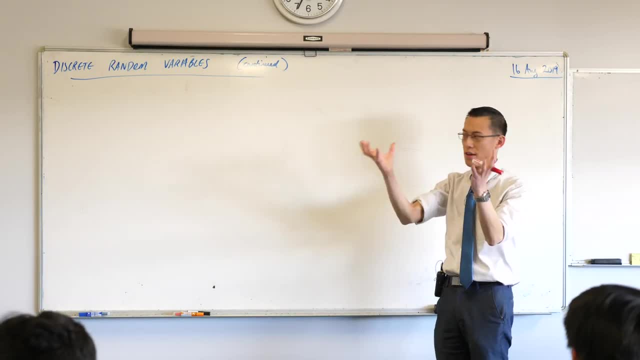 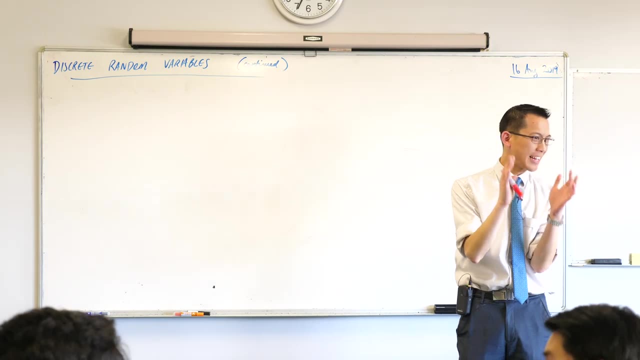 Discrete random variables- This very big, heavy phrase, right? What do we mean by each of these three terms? Hopefully we've been looking at it enough time now that, even if you don't have a technical definition for it, you could explain what each of these bits mean. Let's 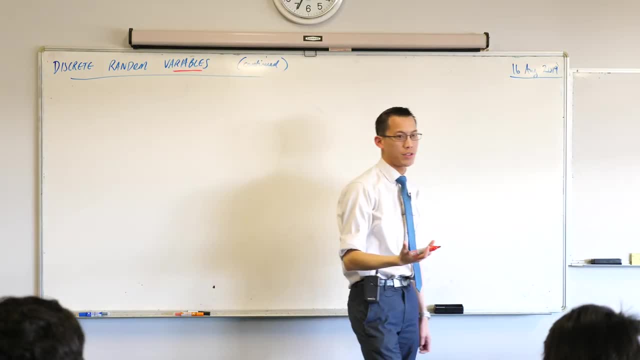 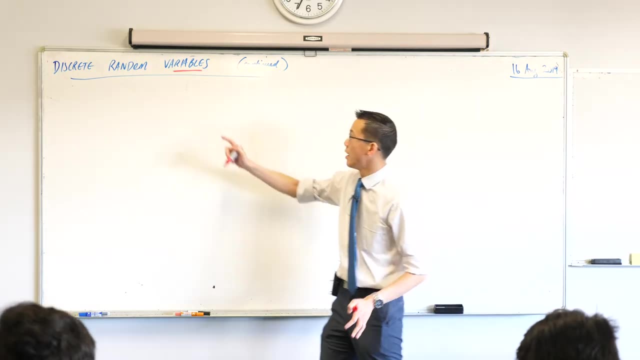 start with the last one. it's the easiest one. When we say variable, why do we say that? Say that again, sorry. Okay, so we have some numbers we want to measure. We put the variable in place of the number mainly because the number can change. right, Variable it can. 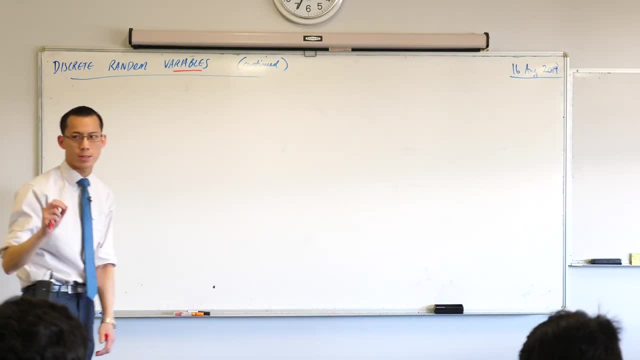 vary. What do we mean? random? This one does have a very specific meaning and it's not the one we usually when we're like, whoa, how random. That's not what this random means. What does this random mean? Anyone want to suggest? Yeah, Will. 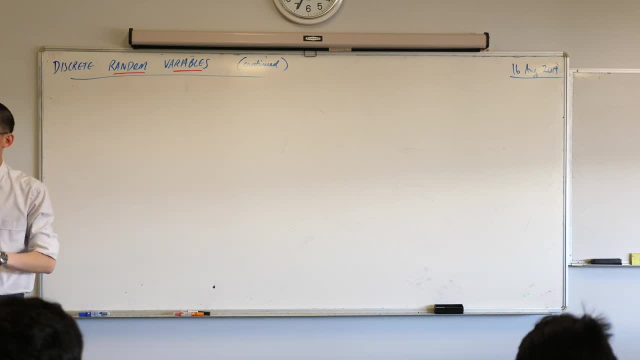 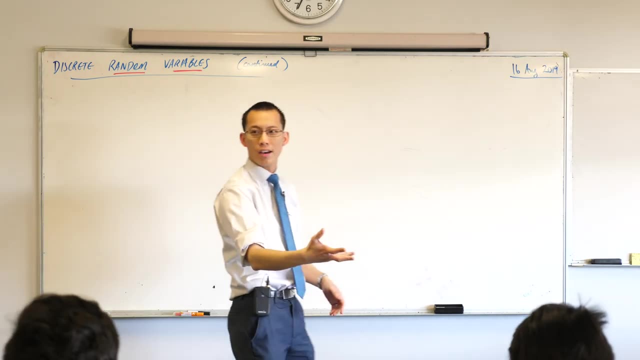 If it's random, it's like multiple outcomes without a bias, Ah, very good. So multiple outcomes. I think the key part of it is the without bias part, right? So if you've got like a loaded die okay, or you're talking to people and they're- 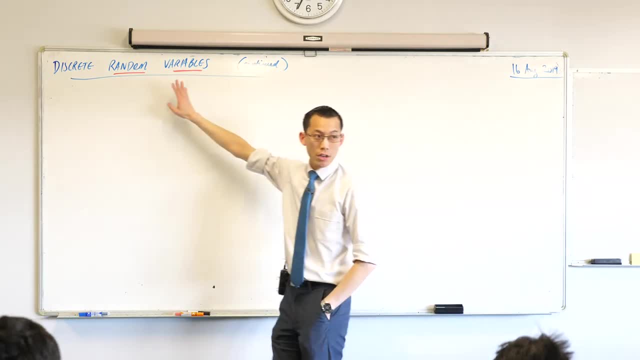 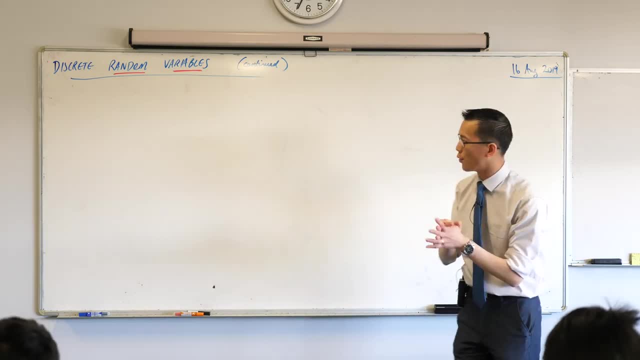 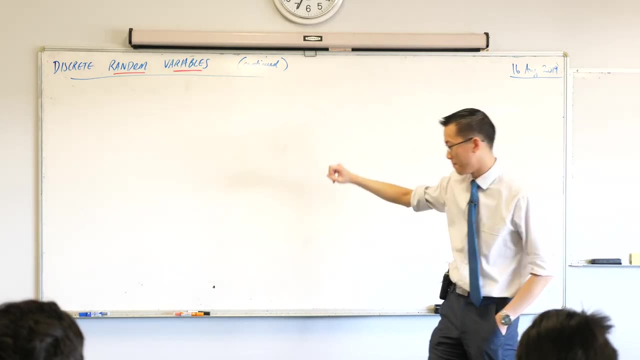 So that's what we mean by that. All options are equally likely, except for whatever the probability density function tells us, and we'll have a look at that in a second. Last one, weirdest one: discrete. What's it mean? Discrete? So mainly it's whole numbers, things. 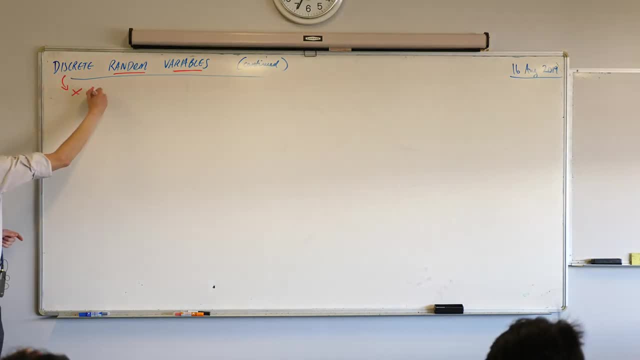 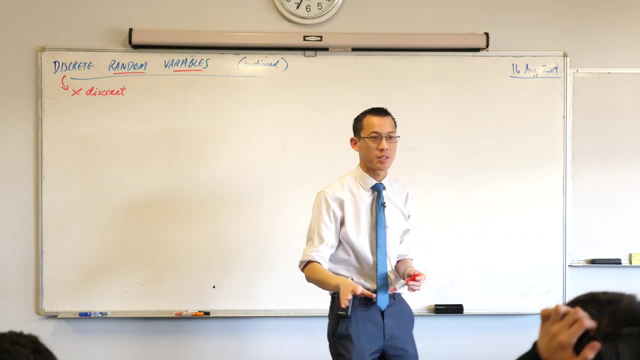 that are separate. okay, By the way, not to be confused with discrete, that has a double E. Does anyone know what that means? Yeah, like shh, do it discreetly, right? So people don't know, okay. Different spelling, same pronunciation. completely different words. 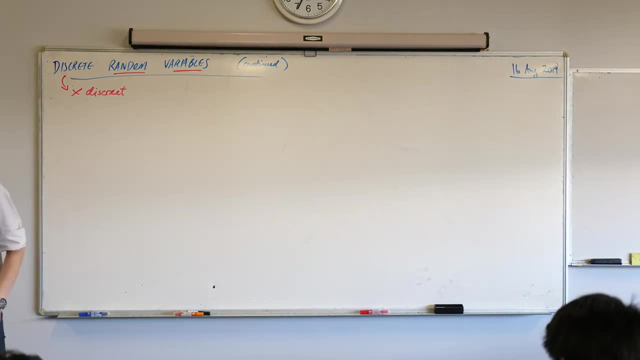 All right, so let's have a look at 20.. You've got that graph in front of you and it shows a discrete probability distribution. So have a look at the bottom axis of the graph. for me, right, One, two, three, four, five, six. So these things cannot mix. If it wasn't a 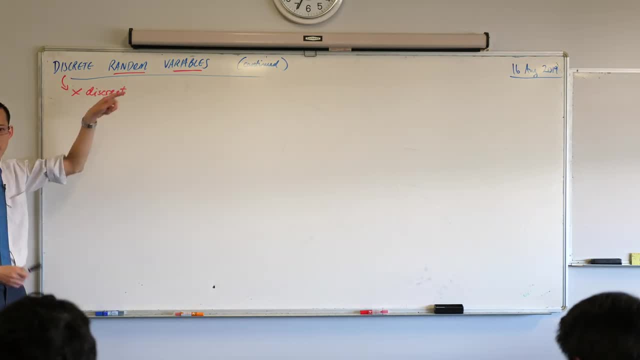 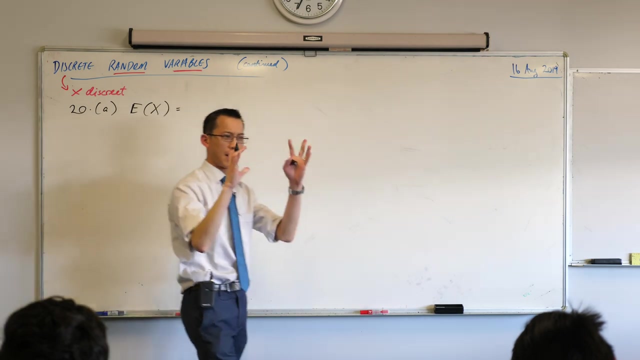 discrete random variable. what kind of random variable would it be if all of the things mixed together? Very good, Continuous is the opposite of discrete, okay, So we want to this distribution. So we've got 20, part A. Let's just remember what's the like fancy. 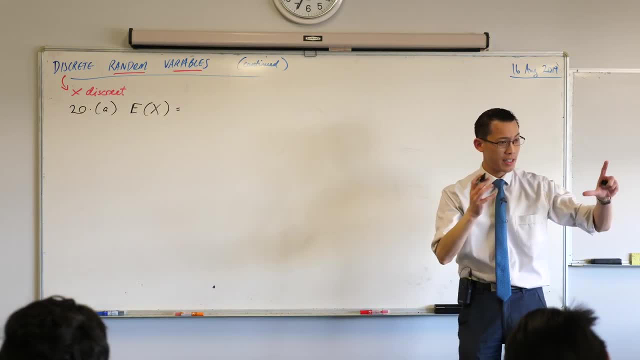 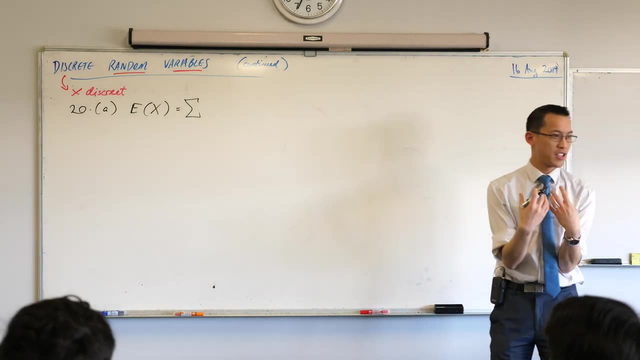 way of saying the calculation for this, We use this weird Greek letter. Does anyone remember which one it was? The sigma. very good, We use the sigma because the Greek letter sigma is equivalent to our S. S stands for what Sum? very good, You're adding up a bunch of. 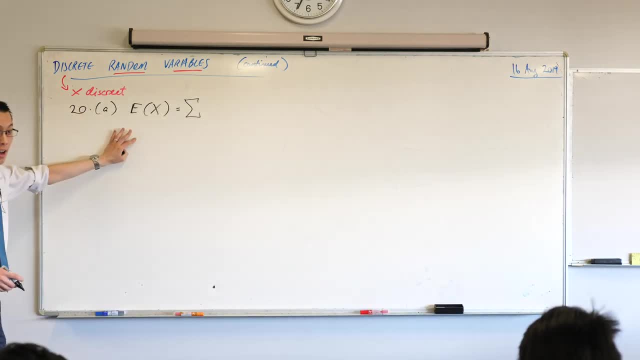 things. What are we adding up To work out expected value? what are we adding up? There's two pieces that go into this, Anyone remember? Yeah, In this example it's just the x values and the y values. Okay, Yeah, very good, So the x values, and we usually write them like so, like the i. 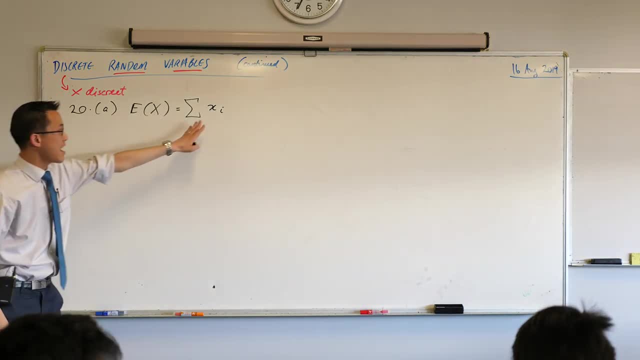 is 0,, 1,, 2,, 3,, 4, etc. So these are the x values. Now the y values. just have a look right. What are the y values here? It's actually not labeled a y axis. We usually call it y. 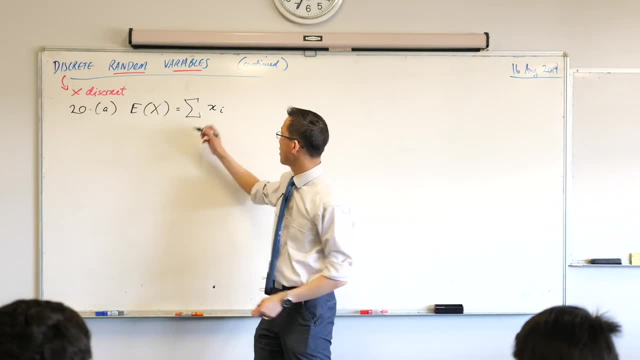 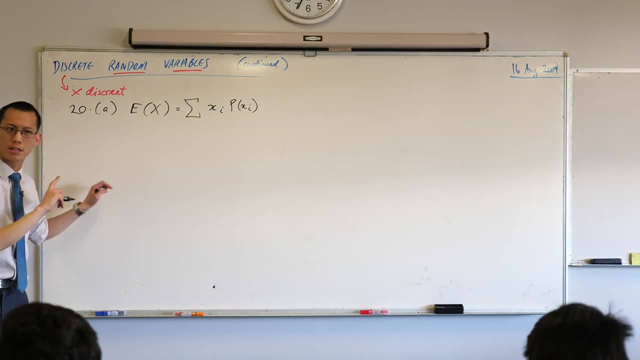 but what is it in this case? P? Yeah, probability P of x, right, So that's going to be the probability of that particular score turning up. There's one thing missing from my sigma notation. Can anyone tell me what it is? It's actually at the beginning When you see this. do you remember When you? 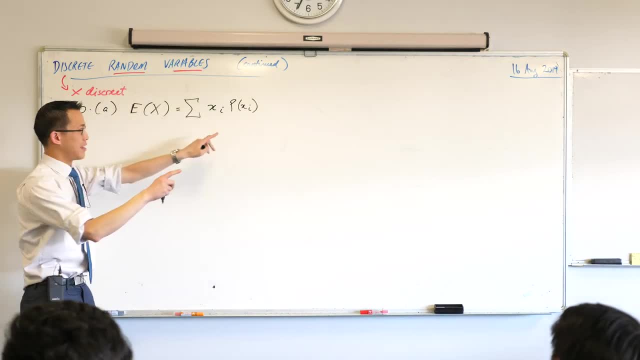 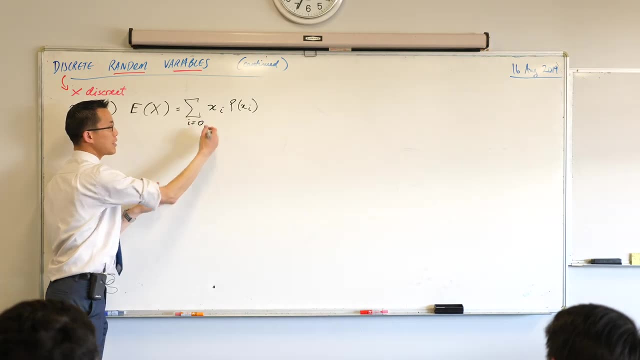 say the sum of a bunch of things. right, You actually have to specify where do you start and where do you end. You would have to specify: i equals. we usually start from 0, and then, in this case, how many scores are there? There's 1,, 2,, 3,, 4 of them, So I'll go from 0 up to. 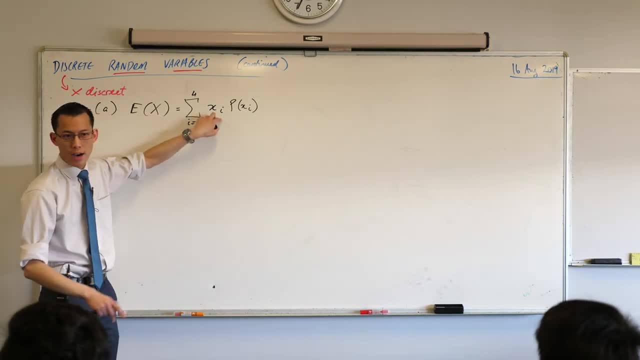 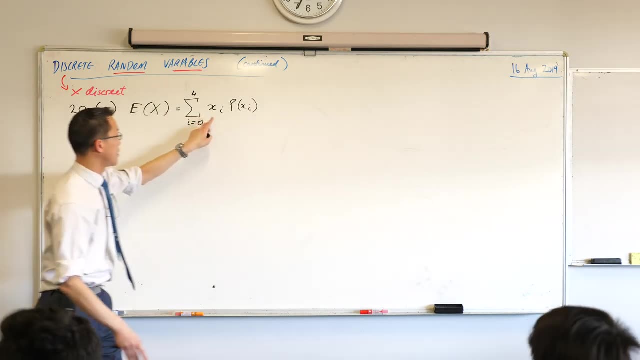 4.. This is not to be confused with what these x values are. are not 0,, 1,, 2,, 3, 4.. What are the values that are relevant for me? Have a look: 2,, 3,, 4, and 5.. Very good, So that's what these numbers are going to be. 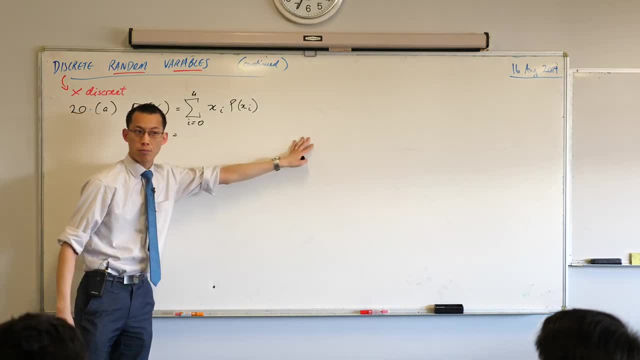 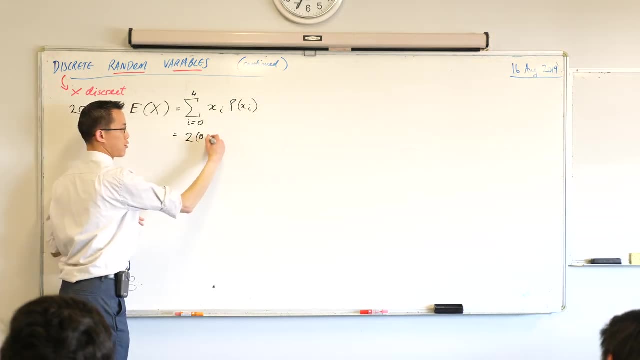 Let's go ahead and actually do this. So we're going to have our 4 different products here. So the first one, you told me it was 2.. What am I going to multiply it by? Thank you, It's probability 0.1.. And then I'm going to add that 2, do this again for. 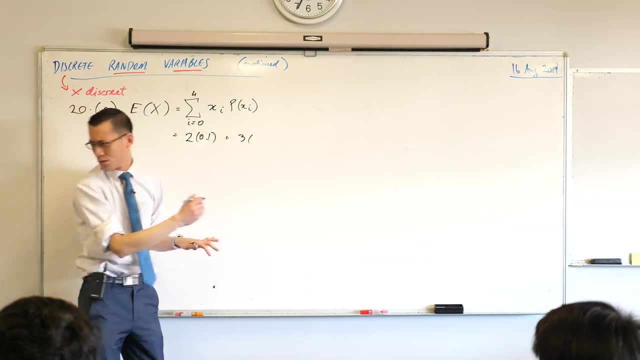 every single one of them along. So I've got 3, is it 0.2?? They just go up in steps, don't they? So that's kind of convenient for us, And now is a good time, if you haven't already. 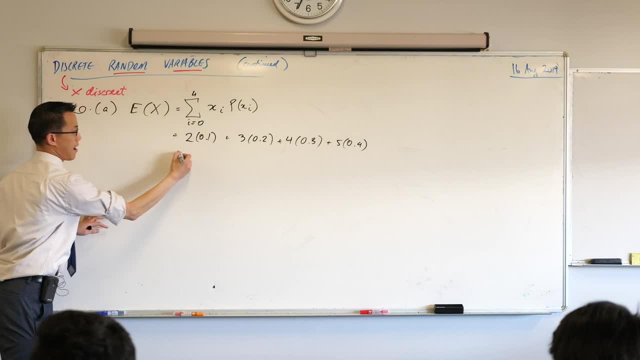 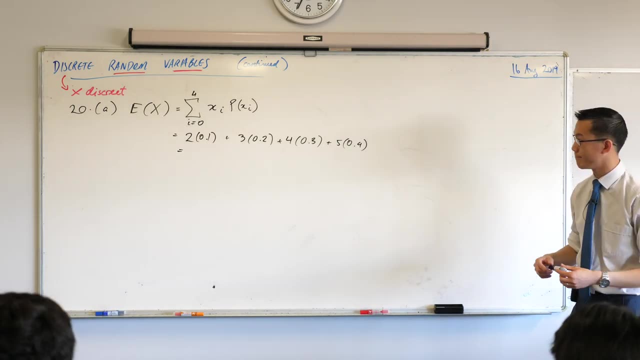 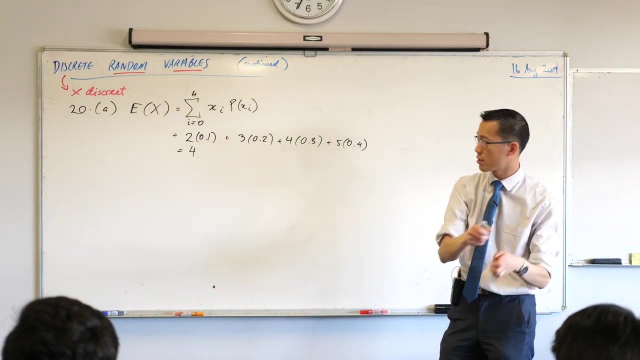 to reach for your calculator because we're going to go ahead and calculate what this expected value is. I'll give you a sec to get to there, Or has anyone already got it? I think I calculated 4 beforehand, So please go ahead. You've got to make sure you do this. 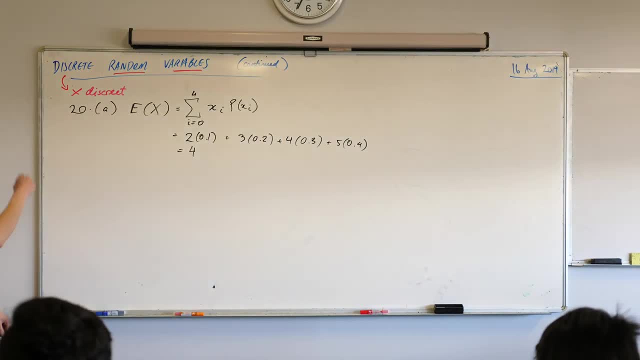 But you should get 4 once you've got that. So this is the expected value. Now, remember it, because we're going to turn the page and use this to answer the next question. So have a look over. I'm just going to suggest. if there's two of you who can see this, maybe one person. 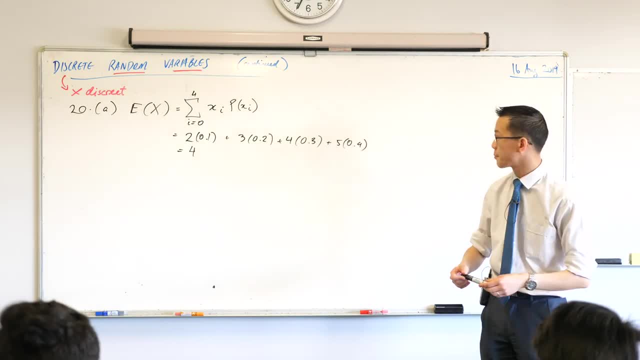 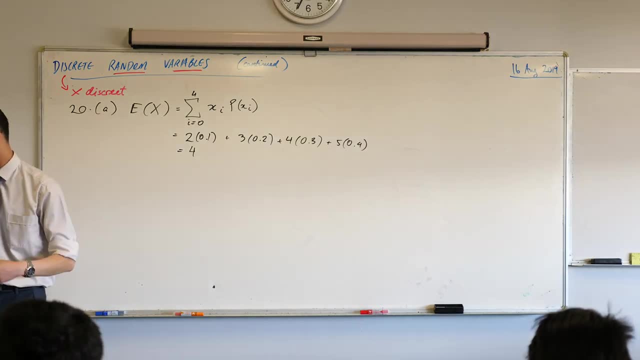 turn their page. the other person: stay on the original page, because we'll also need that Part B. what does it ask? It's a bit of a mouthful. Would you expect the median to be greater than, less than or equal to the expected value of this distribution? Okay, there's. 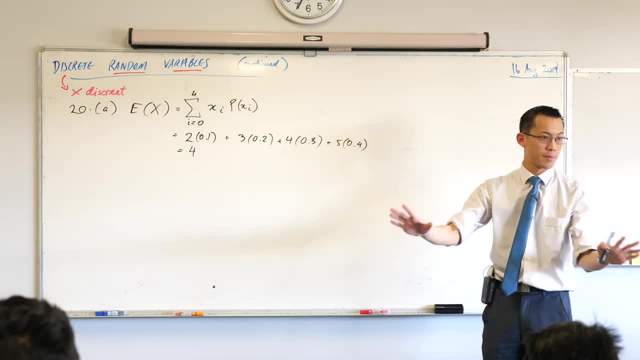 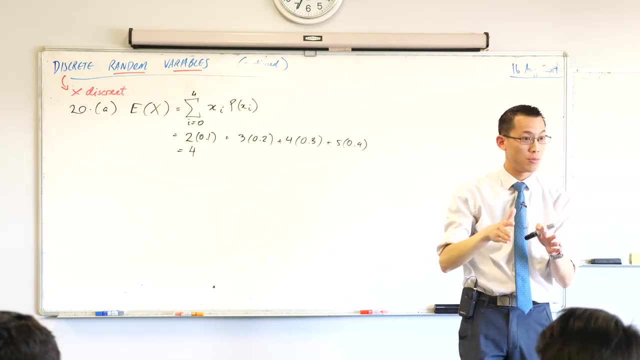 a lot there. right, Put it in your hand if and if no one puts up their hands, that's fine. but I just want to know, Put it in your hand if you could say I know how to find the median. that's the first thing you're asking for in this distribution. 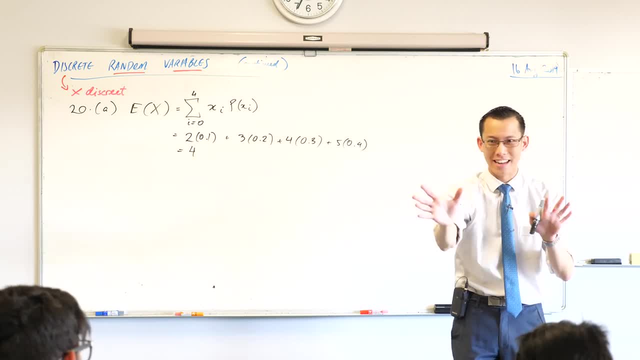 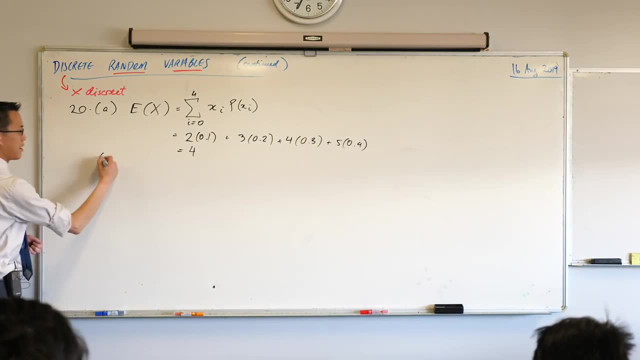 Any takers? Yeah, I'm not going to ask you, I just want an indication. Alright, that's fine. Okay, thank you, Let's all try and work out how this is calculated. What is median? This is part B. It's the middle number, the middle value, right? So what we're looking? 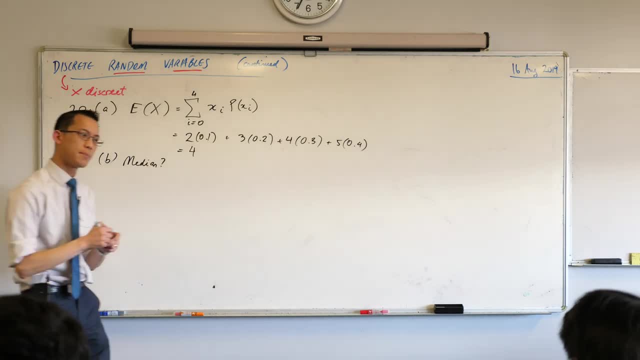 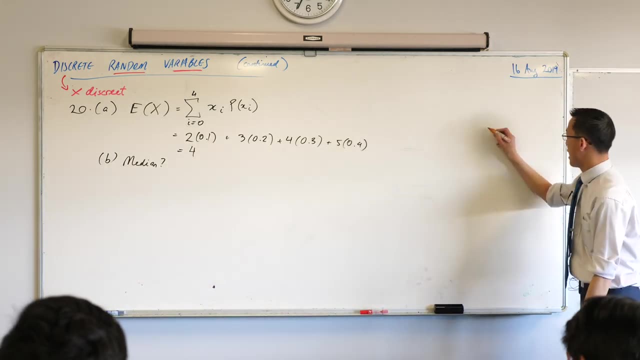 for is: where does the median occur? Now, it's a bit tricky when you've got a probability distribution, because normally we would say something like there's five people right And you want to say, okay, which one has the median height? So what would you do? You would 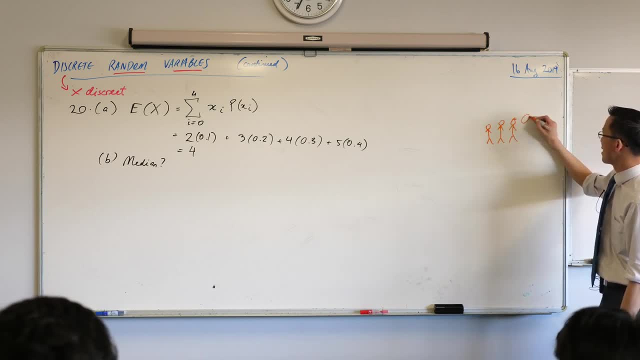 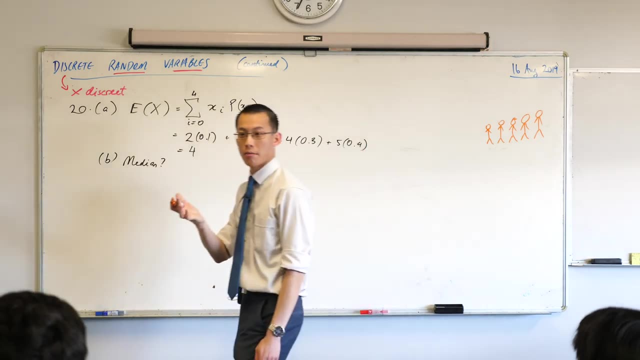 arrange them. let's give them a tall haircut. you'd arrange them somewhat. this guy just has a big head, that's why they're taller. you'd arrange them in height order, right, And then you just say which one's the middle one? okay, Now have a look at this probability. 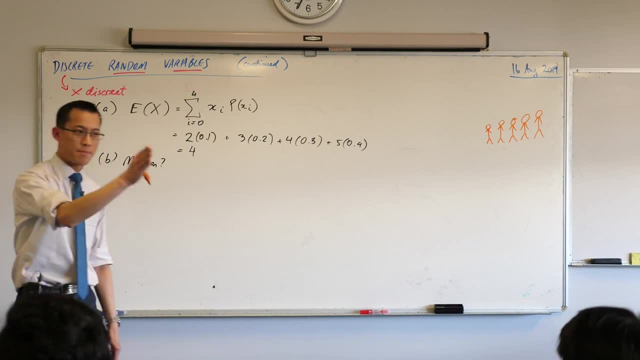 graph. there's no like bunch of people or bunch of items and then you can just count along, right, All we've got is probabilities. okay, But we can work this out nonetheless by calculating. and where you've got part B written there, can I ask you to write down? 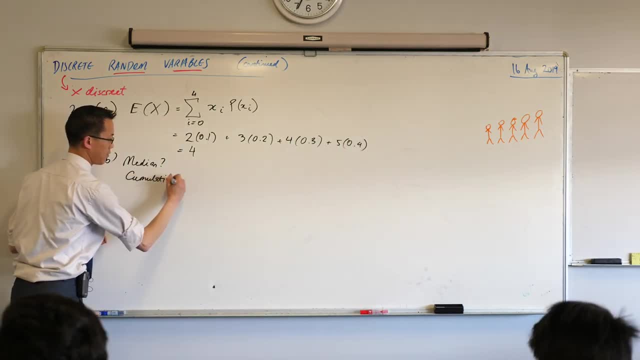 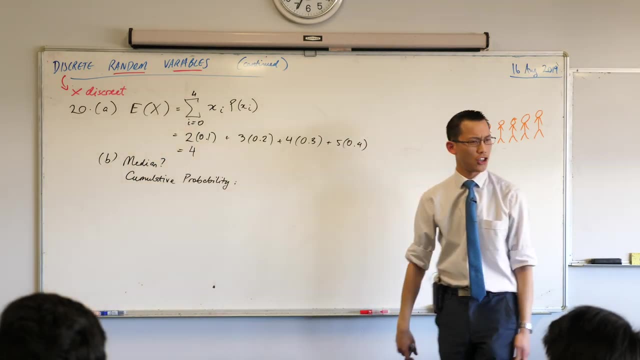 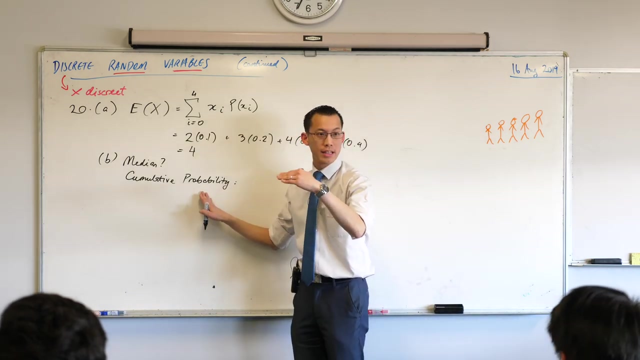 the phrase cumulative, cumulative- Okay, Cumulative probability. So this is very similar to cumulative frequency, If you remember calculating that all the way back in like year seven and eight. what we're going to do is we're going to add up the probabilities and let them accumulate as we go further along. 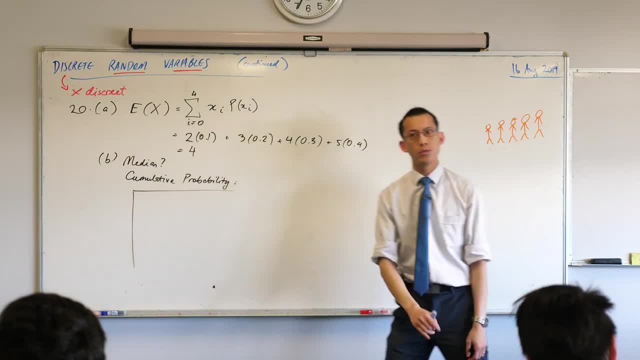 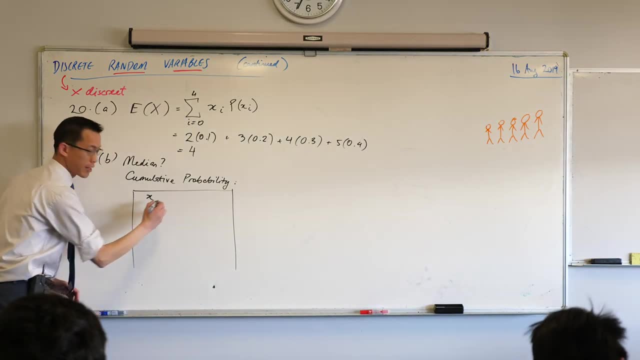 okay, So draw me a little table, and on our table we will need one, two, three columns. They don't need to be huge, though. three columns. The first column is going to be our particular X values. So if you already told me what they were, they are two, three, four and five. okay, 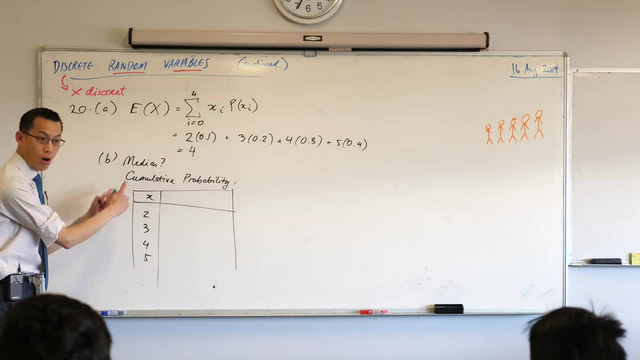 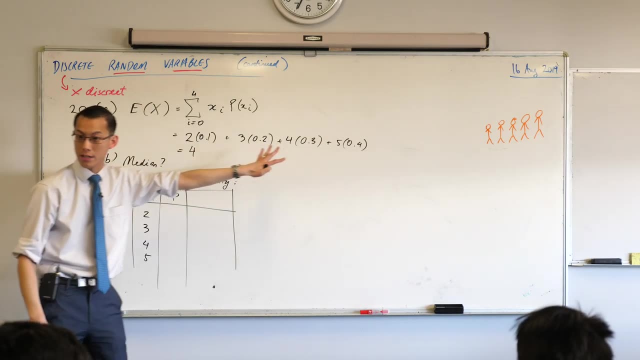 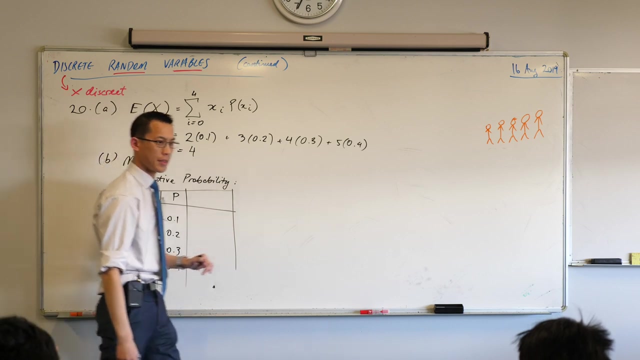 In this table we're also going to have the probability of those X values. So I'll just write P for probability and we have that written in our expected value calculation. Yeah, so it's zero point one, zero point two, and so on. Okay, Now, this last one is the. 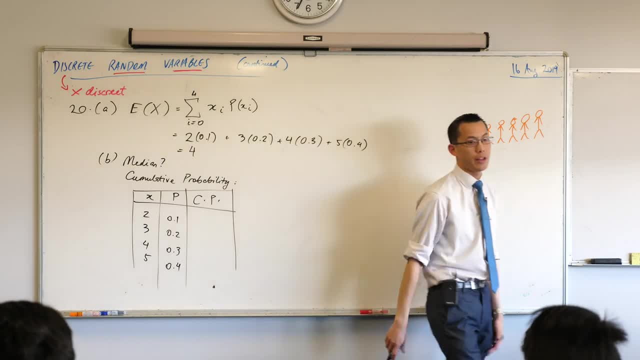 cumulative probability. So just to get this slide. Okay, So that was the cumulative probability. So just to get the cumulative probability. So just to get the cumulative probability. So let's say we're like, with cumulative frequency we're just going to add everything as we progress down the table. so 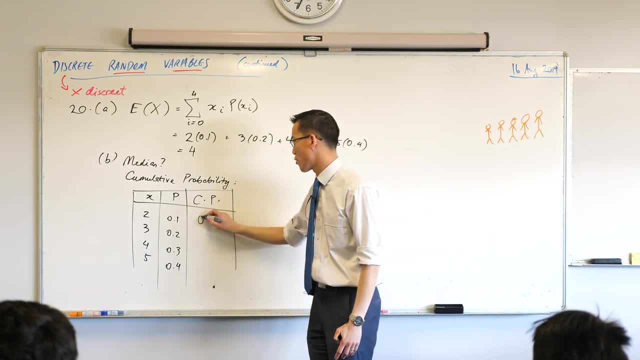 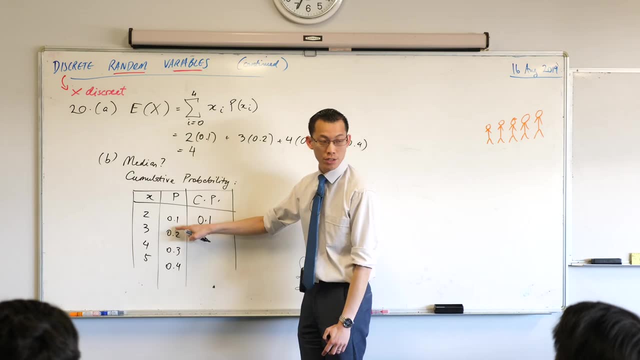 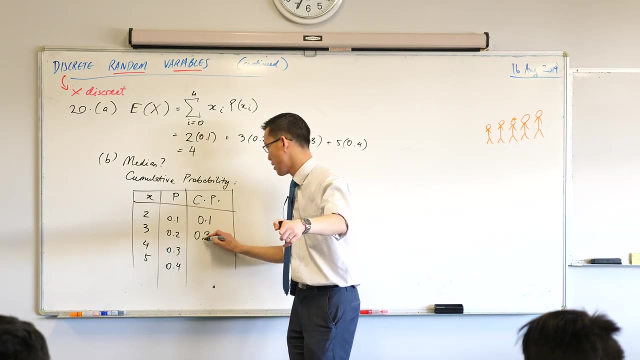 for the first row. i only have one probability to add. it's there 0.1. okay, as i write the next one, i'm including all of the probabilities before, so it's 0.2 and all the previous ones. so what will the cumulative probability be here? 0.3. that's it now. at this point, i'm going to add. 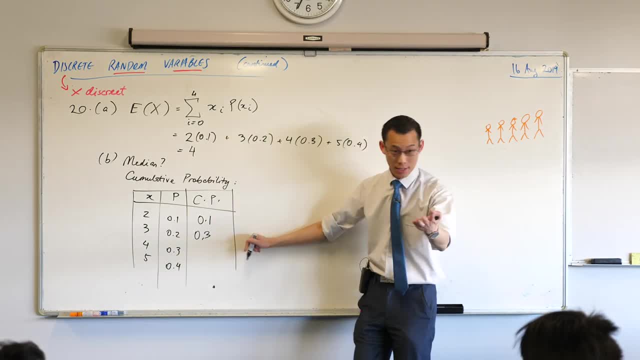 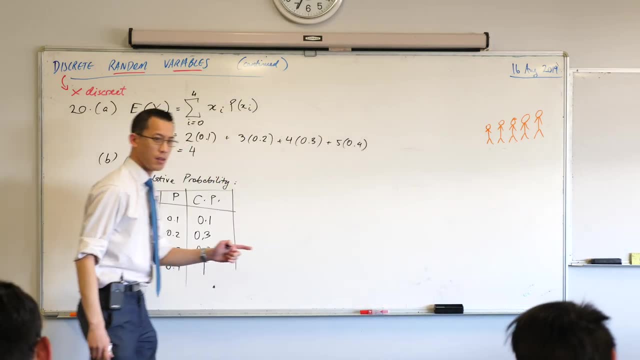 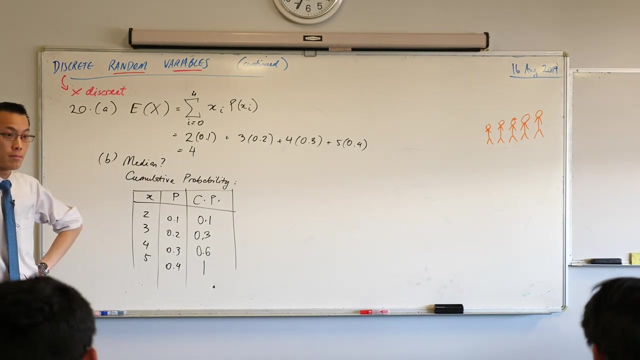 next probability and all the previous ones, so 0.6. very good, and then the last one gives me one, which it should. why is that? it's it's. what does one mean in this context? yeah, it better add up to one. that means i've got a comprehensive list of all the things that can. 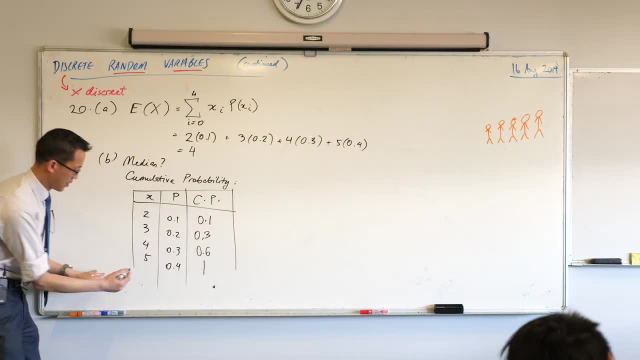 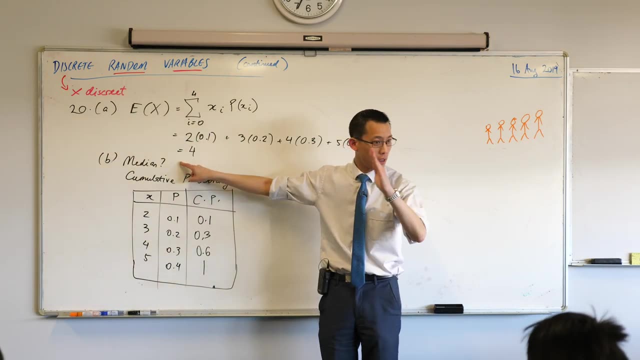 possibly happen. the total probability is one if i add everything up together. okay, so there's the end of our table. now how do we use this? the median is supposed to increase from and for. The median is supposed to come, like you told me, halfway, like in the middle right. 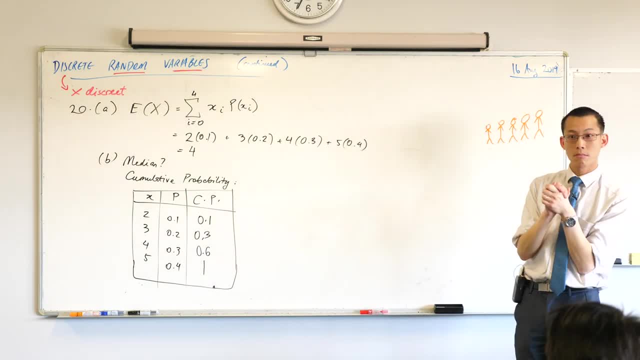 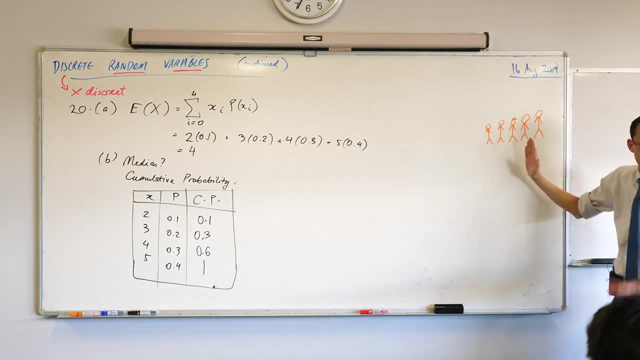 So what would the middle probability be? It would be 0 point. think carefully. like halfway through, like the position would be 0.5 the way through. Does that make sense? If the final person is 1, then the middle person should be 0.5.. 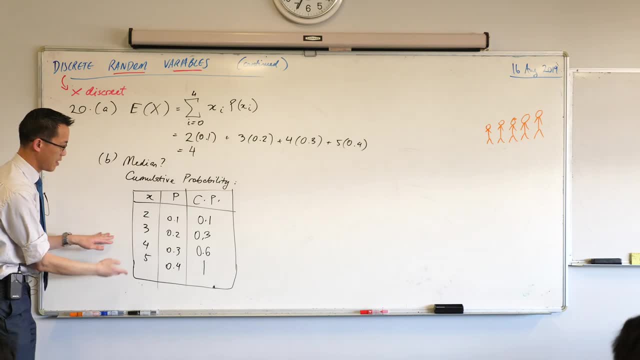 So what I'm going to do? because it's discrete, I have to go up in steps, right. So let me ask- humor me okay, By this value, have I gotten to 0.5 yet? No, I haven't. 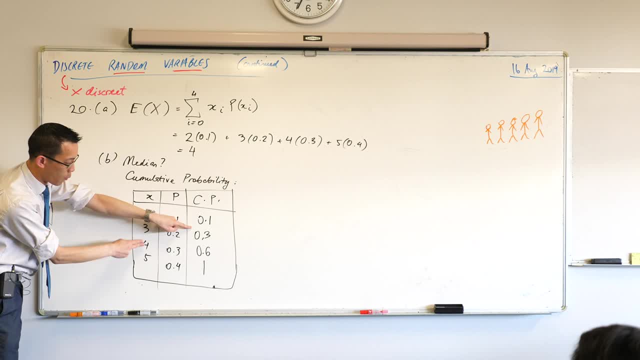 By this value. have I gotten to 0.5 yet? No, I haven't. But once I cross into here, somewhere in here, I get to 0.5.. In fact, I go past it, don't I? 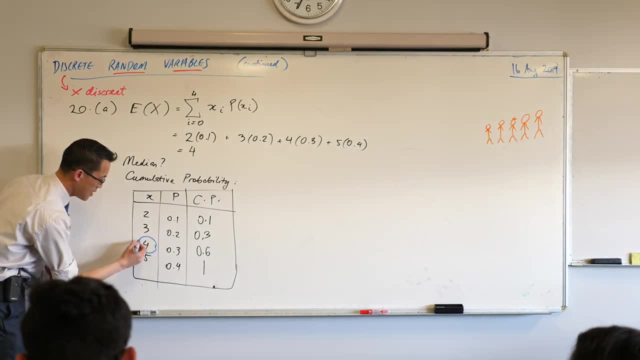 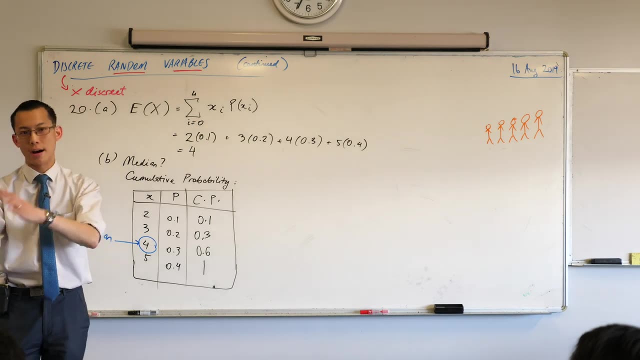 So this value here, this is the median. It's wherever. what's the first moment, the first instance that you pass that 0.5 threshold? Might be worth jotting that down: It's when we pass, We pass, the cumulative probability being 0.5.. 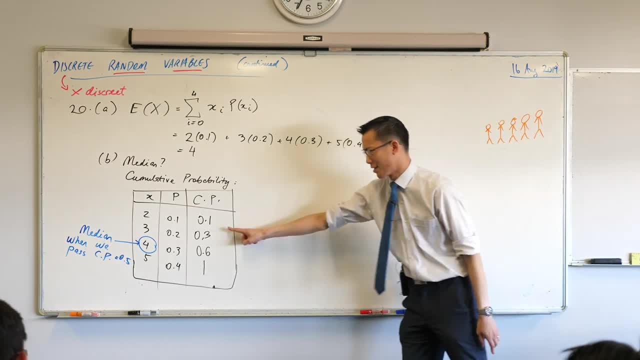 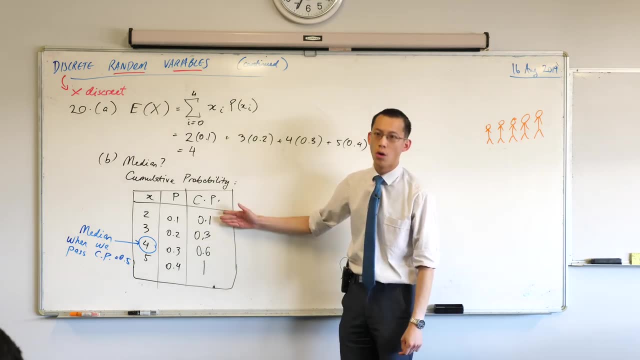 It's a bit weird that it isn't exactly 0.5.. You're like it's not this one and it's not that one. The whole point of discrete random variables is that you can't say it's in between. You're one or the other, okay. 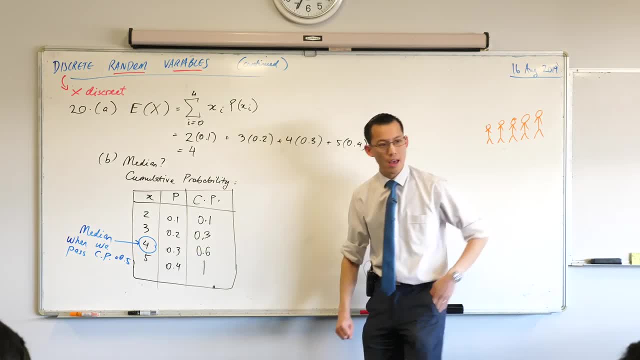 Because you haven't gotten to it here. it only happens on the next one. Can we use this to answer our question? Look back at the question. It's a bit of a mouthful right. It says: I actually have the book here. 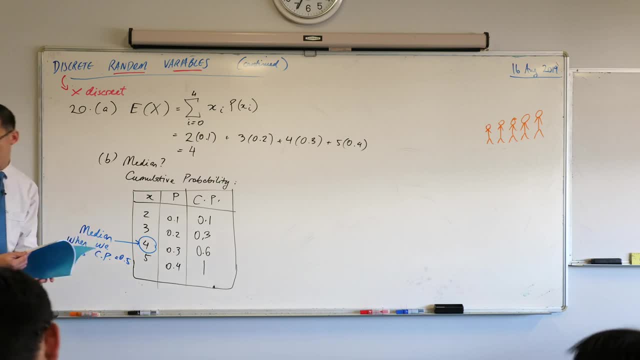 Oops, where'd it go? Would you expect the median to be greater than, less than or equal to the expected value? What's our answer? It is exactly equal to. We worked out expected value here, and then here's our median. 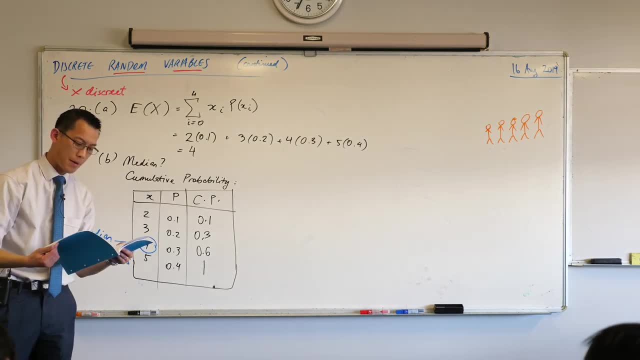 So far, so good. You can say: you can write down if you like, it is equal, It is equal.